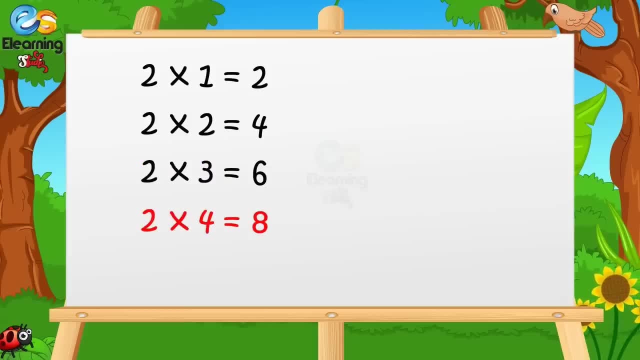 Two, threes are six. Two threes are six. Two fours are eight. Two fours are eight. Two fives are ten. Two fives are ten. Two sixes are twelve. Two sixes are twelve. Two sevens are fourteen. Two sevens are fourteen. 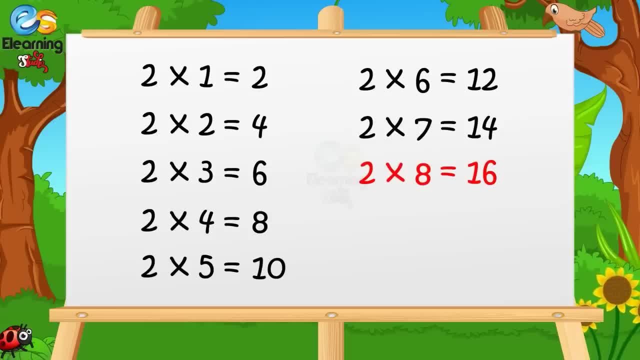 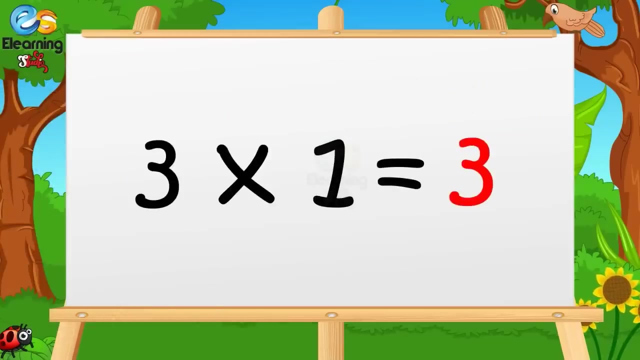 Two eights are sixteen. Two eights are sixteen. Two nines are eighteen. Two nines are eighteen. Two tens are twenty. Two tens are twenty. Table of three. Three ones are three. Three ones are three. Three twos are six. Three twos are six. 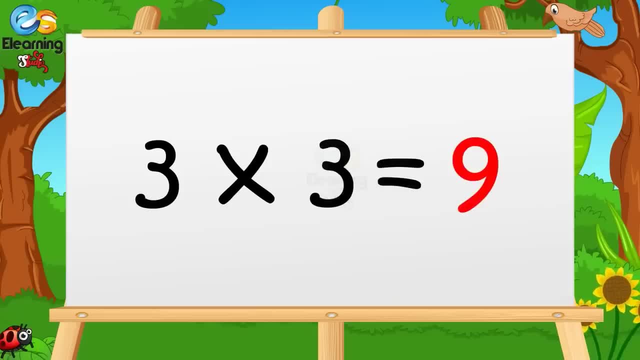 Three threes are nine. Three threes are nine. Three fours are twelve. Three fours are twelve. Three fives are fifteen. Three fives are fifteen. Three sixes are eighteen. Three sixes are eighteen. Three sevens are twenty-one. Three sevens are twenty-one. 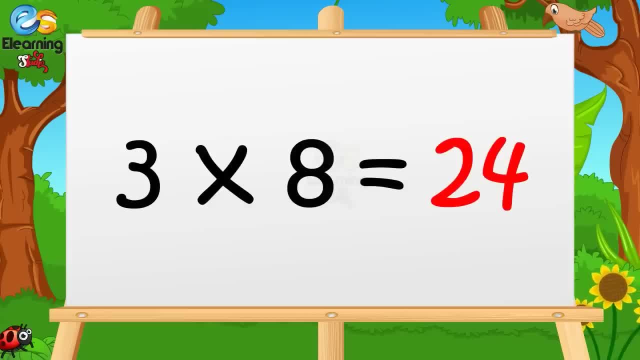 Three eights are twenty-four. Three eights are twenty-four. Three nines are twenty-seven. Three nines are twenty-seven. Three tens are thirty. Three tens are thirty. Three ones are three. Three ones are three. Three twos are six. Three twos are six. 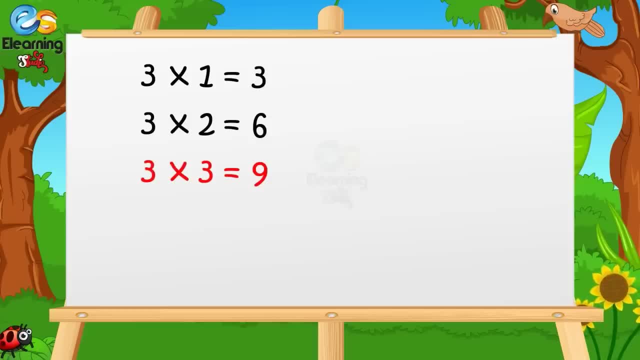 Three threes are nine. Three threes are nine. Three fours are twelve. Three fours are twelve. Three fives are fifteen. Three fives are fifteen. Three sixes are eighteen. Three sixes are eighteen. Three sevens are twenty-one. Three sevens are twenty-one. 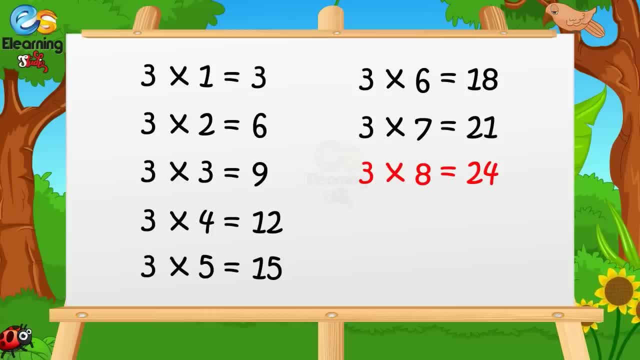 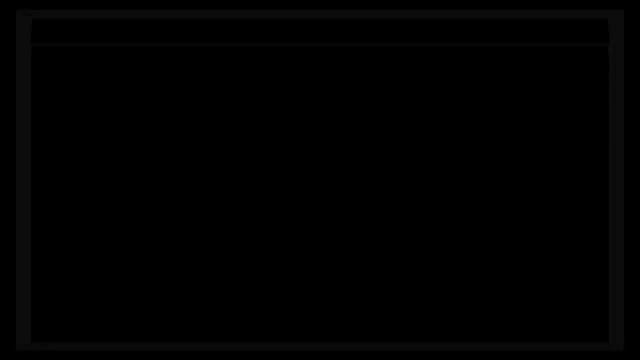 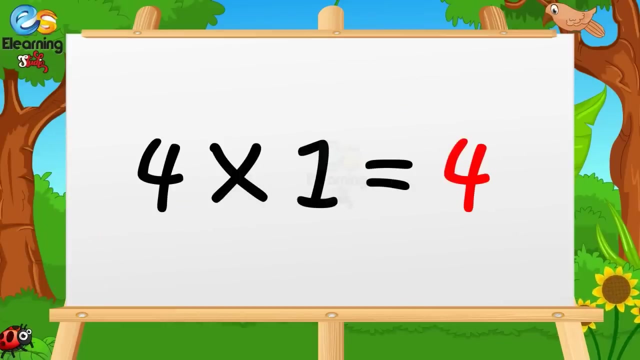 Three eights are twenty-four. Three eights are twenty-four. Three nines are twenty-seven. Three nines are twenty-seven. Three tens are thirty. Three tens are thirty. Four ones are four. Four ones are four. Four twos are eight. Four twos are eight. 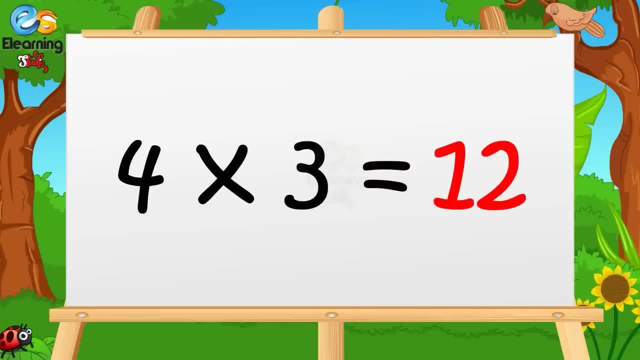 Four threes are twelve. Four threes are twelve. Four fours are sixteen. Four fours are sixteen. Four fives are twenty Four. fives are twenty Four. sixes are twenty-four. Four sixes are twenty-four. Four sevens are twenty-eight. Four sevens are twenty-eight. 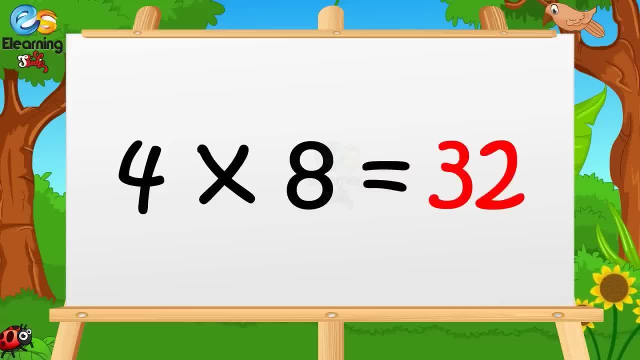 Four eights are thirty-two. Four eights are thirty-two. Four nines are thirty-six. Four nines are thirty-six. Four tens are forty. Four tens are forty. Four ones are four. Four ones are four. Four twos are eight. Four twos are eight. 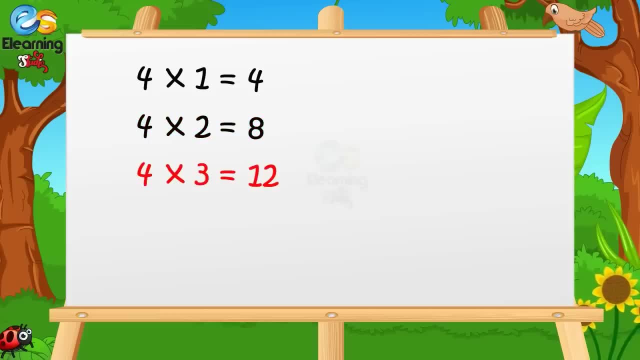 Four threes are twelve. Four threes are twelve. Four fours are sixteen. Four fours are sixteen. Four fives are twenty Four. fives are twenty Four. sixes are twenty-four. Four sixes are twenty-four. Four sevens are twenty-eight. Four sevens are twenty-eight. 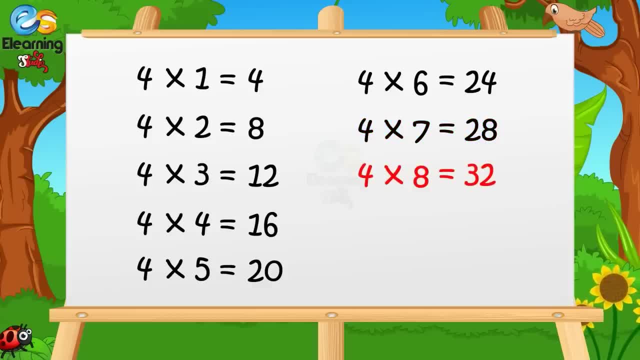 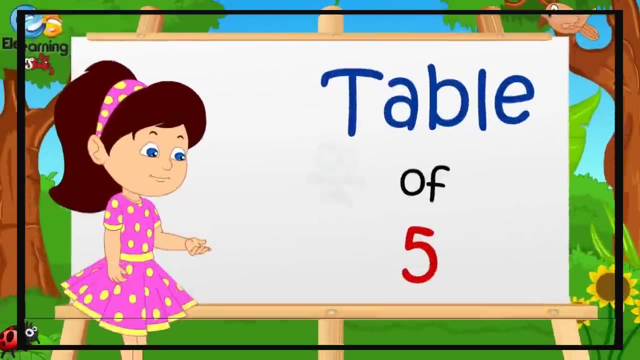 Four eights are thirty-two. Four eights are thirty-two. Four nines are thirty-six. Four nines are thirty-six. Four tens are forty. Four tens are forty. Table of Five. Five ones are five. Five ones are five. 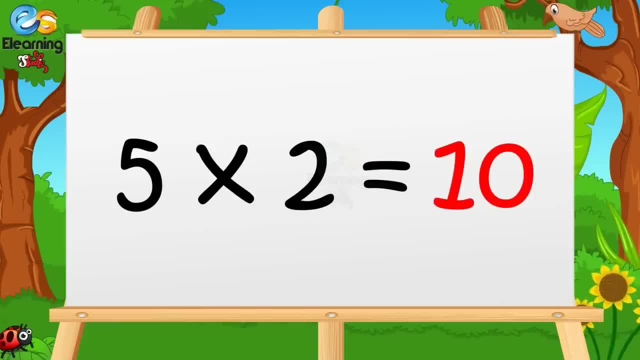 Five twos are ten. Five twos are ten. Five threes are fifteen. Five threes are fifteen. Five fours are twenty Five. fours are twenty Five. fives are twenty-five. Five fives are twenty-five. Five sixes are thirty. Five sixes are thirty. 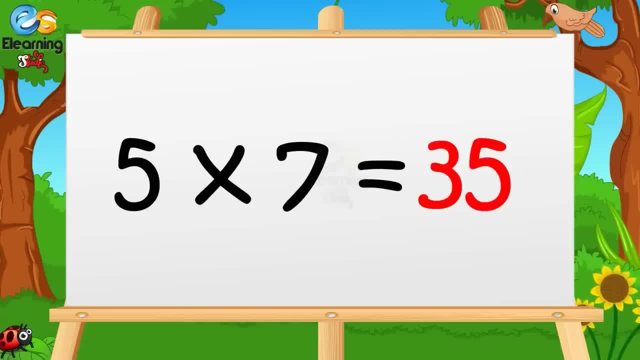 Five sevens are thirty-five. Five sevens are thirty-five. Five eights are forty Five. eights are forty Five. nines are forty-five. Five nines are forty-five. Five tens are fifty Five. tens are fifty. Five ones are five. Five ones are five. 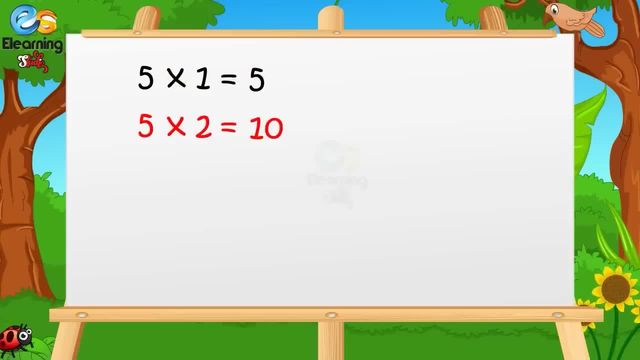 Five. twos are ten. Five twos are ten Five. threes are fifteen. Five fours are twenty Five. fours are twenty Five. fives are twenty-five. Five fives are twenty-five. Five sixes are thirty Five. sixes are thirty Five. sevens are thirty-five. 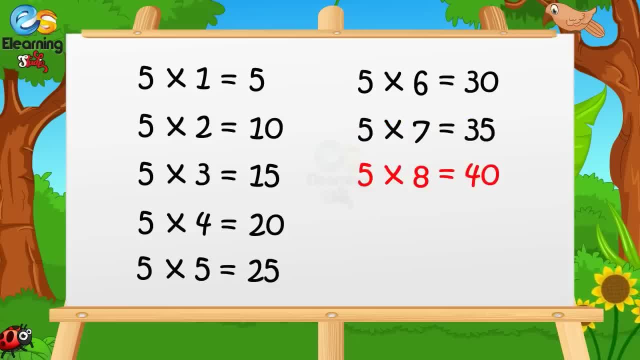 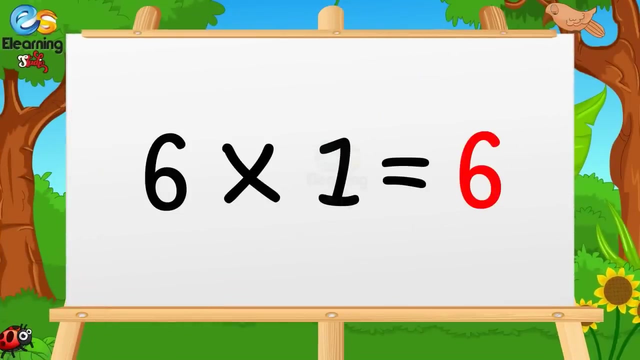 Five sevens are thirty-five. Five eights are forty Five. eights are forty Five. nines are forty-five. Five nines are forty-five. Five tens are fifty. Table of Six. Six ones are six. Six ones are six. 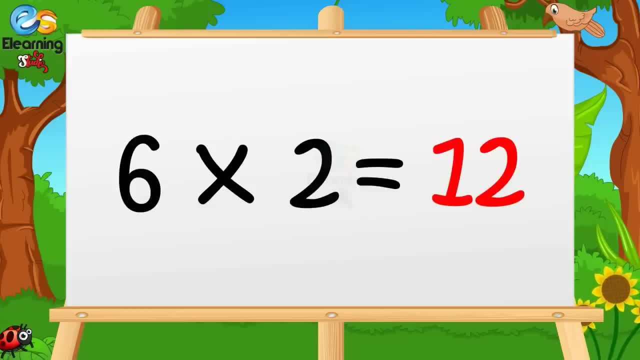 Six, twos are twelve. Six, twos are twelve. Six, threes are eighteen. Six, threes are eighteen. 3s are 18, 6, 4s are 24, 6, 4s are 24, 6, 5s are 30, 6, 5s are 30, 6, 6s are 36, 6, 6s are 36, 6, 7s are 42, 6. 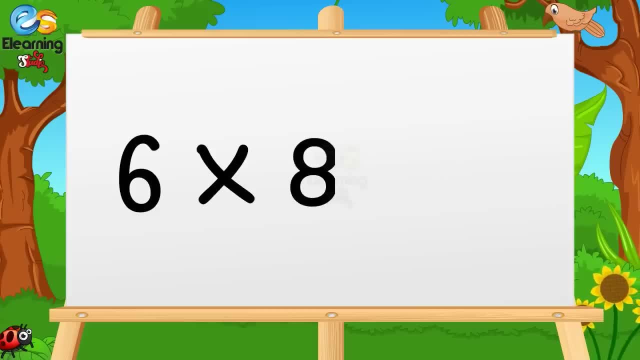 7s are 42, 6 8s are 48, 6 8s are 48, 6 9s are 54, 6 9s are 54, 6 10s are 60, 6 10s are 60. 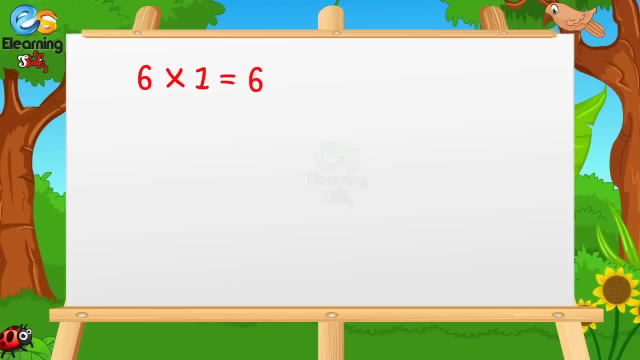 6. 1s are 6, 6, 1s are 6, 6, 2s are 12, 6, 2s are 12. 6, 3s are 18. 6, 3s are 18. 6, 4s are 24. 6, 4s are 24. 6, 5s are 30. 6, 5s are 30, 6, 6s are 36. 6, 6s are 36, 6, 7s are 42. 6, 7s are 42, 6, 7s are 42. 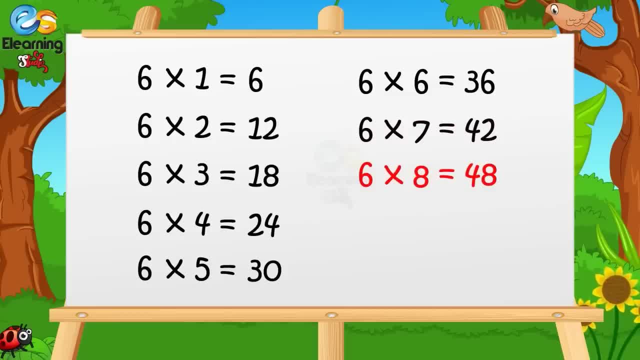 6 8s are 48. 6 8s are 48. 6 9s are 54. 6 9s are 54. 6 10s are 60. 6 10s are 60, 6 10s are 60. 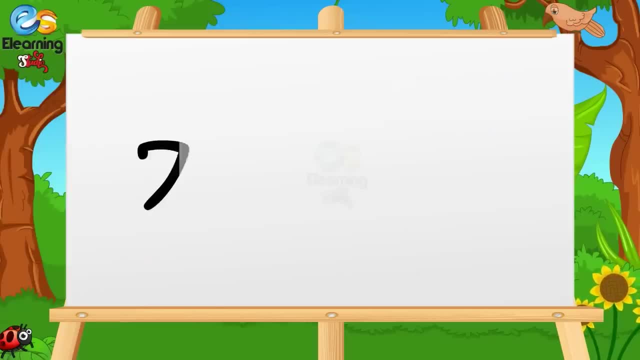 Table of 7. 7 1s are 7. 7 1s are 7. 7 2s are 14. 7 2s are 12. 2s are 14, 7 3s are 21,. 7 3s are 21,. 7 4s are 28,. 7 4s are 28,. 7 5s are 35, 7 5s are. 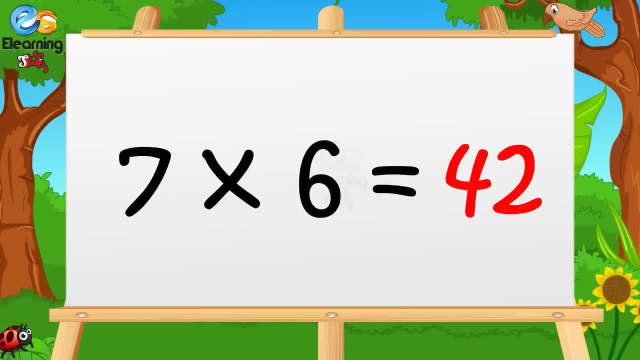 35,. 7- 6s are 42,. 7- 6s are 42,. 7- 7s are 49,. 7- 7s are 49,. 7- 8s are 56,. 7- 8s are 56,. 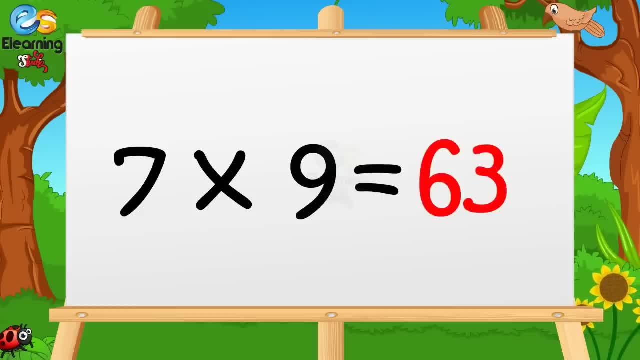 7 9s are 63,. 7 10s are 70,, 7 10s are 70,. 7 1s are 7, 7 1s are 7,. 7 2s are 14,. 7 2s are 14, 7 3s are 21,. 7 3s are 21,. 7 4s are. 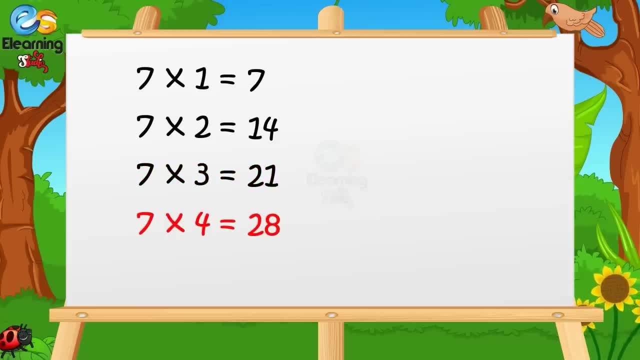 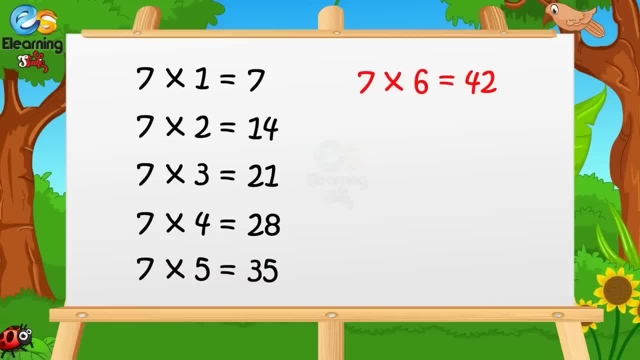 6s are 42,. 7. 6s are 42, 7. 7s are 49,. 7. 7s are 49, 7. 8s are 56,. 7. 8s are 56, 7. 9s are: 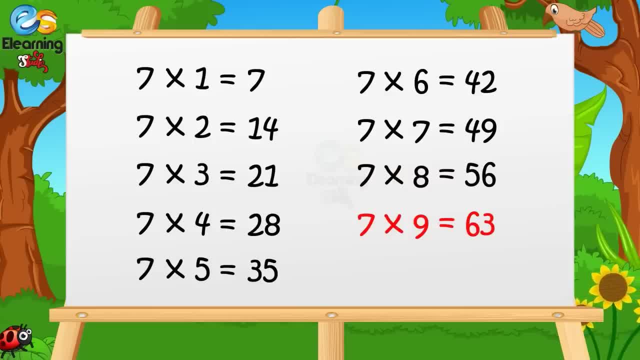 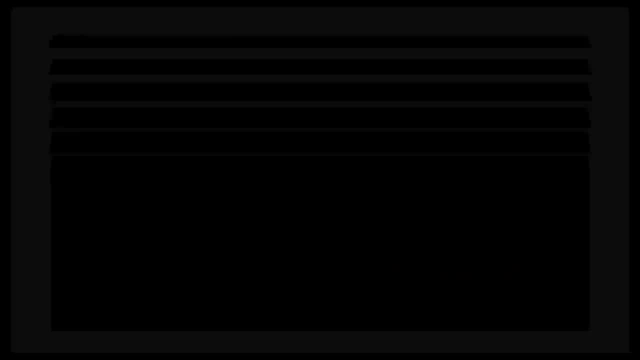 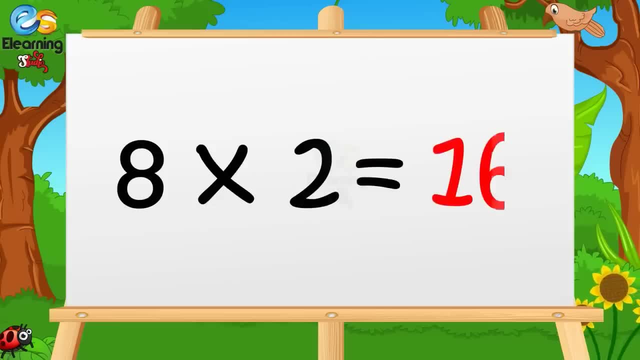 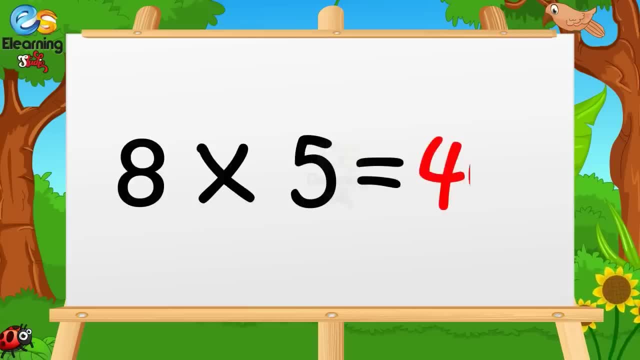 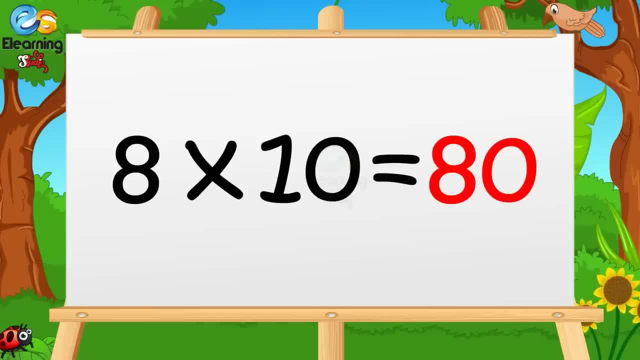 8 10s are 80,. 8 10s are 80,. 8 1s are 8,. 8 1s are 8,. 8 2s are 16,. 8 2s are 16,. 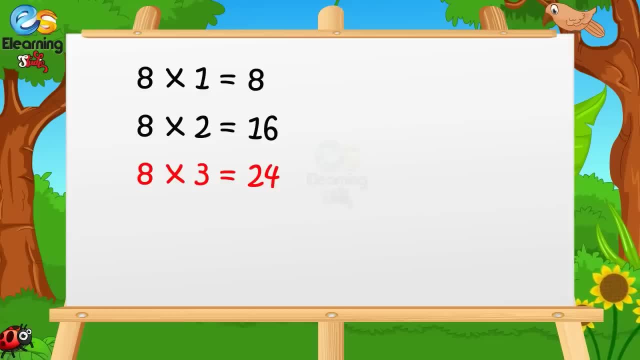 8 3s are 24,. 8 3s are 24,. 8 4s are 32,. 8 4s are 32,. 8 5s are 32,. 8 5s are 32,. 8 4s are 32,. 8 5s are 32,. 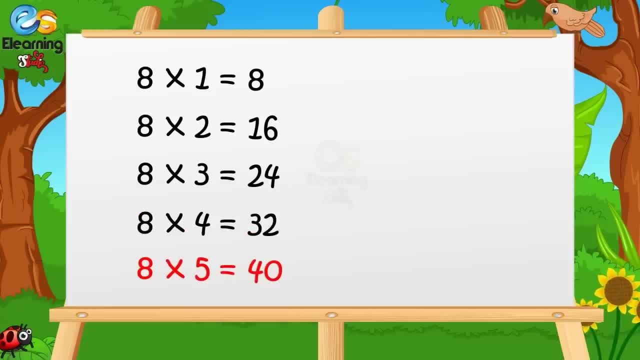 8 1s are 40,. 8- 5s are 40,. 8- 6s are 48,. 8- 6s are 48,. 8- 7s are 56,. 8- 7s are 56,. 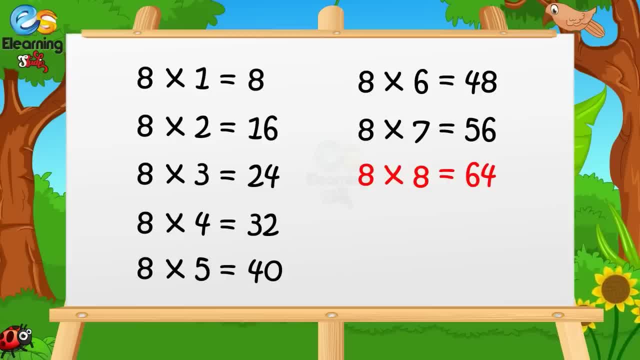 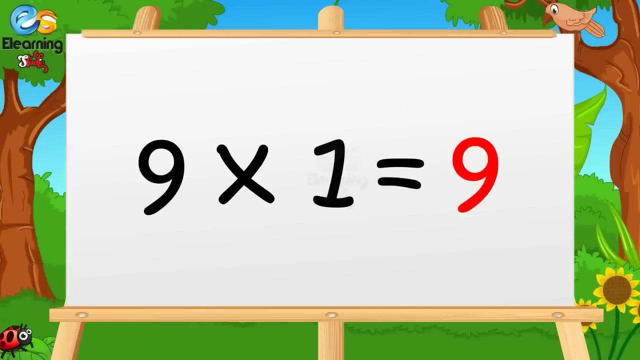 8. 8s are 64,. 8. 9s are 72,, 8. 10s are 80,. table of nine. nine ones are nine. nine ones are nine. nine twos are eighteen. nine twos are eighteen. nine threes are twenty seven. nine threes are 27. nine fours are 36. nine fours are 36. 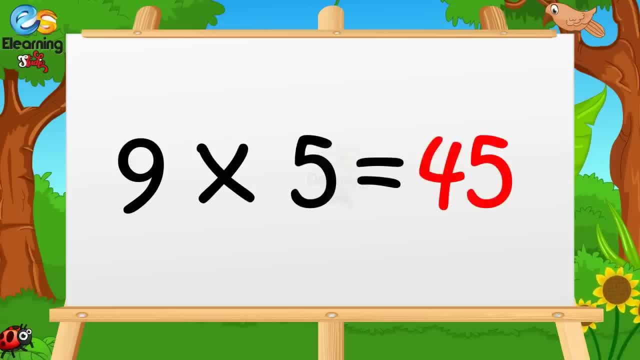 nine fives are 45. nine fives are 45. nine six of 54. nine. six of 54. nine sevens are 63. Nine sevens are sixty-three. Nine eights are seventy-two. Nine eights are seventy-two. Nine. nines are eighty-one. Nine tens are ninety. 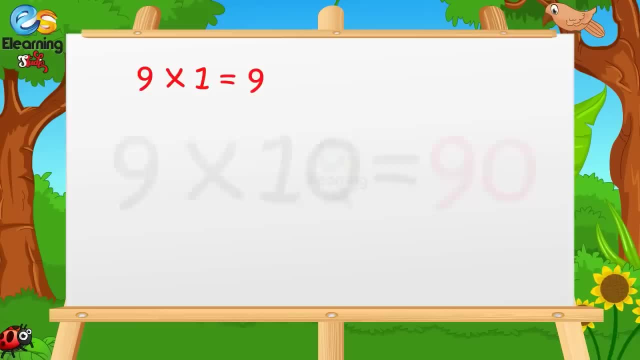 Nine ones are nine. Nine twos are eighteen. Nine threes are twenty-seven. Nine threes are twenty-seven. Nine fours are thirty-six. Nine fours are thirty-six. Nine fives are forty-five. Nine fives are forty-five. Nine sixs are fifty-four. 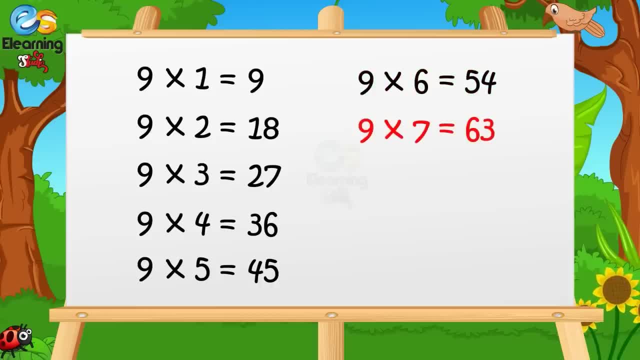 Nine sixs are fifty-four. Nine sevens are sixty-three. Nine sevens are sixty-three. Nine eights are seventy-two. Nine eights are seventy-two. Nine nines are eighty-one. Nine nines are eighty-one. Nine tens are ninety. Nine tens are ninety. 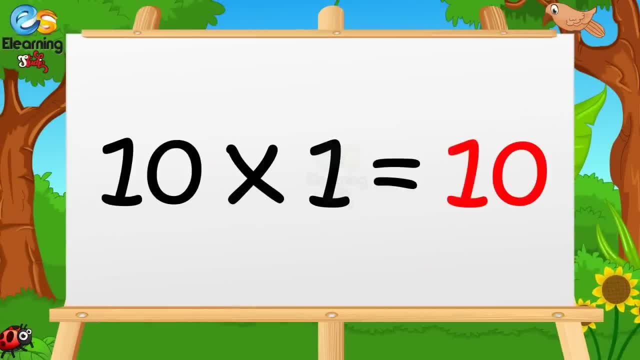 Table of ten. Ten ones are ten. Ten ones are ten. Ten twos are twenty. Ten twos are twenty. Ten threes are thirty. Ten threes are thirty. Ten fours are forty. Ten fours are forty. Ten. fives are fifty. 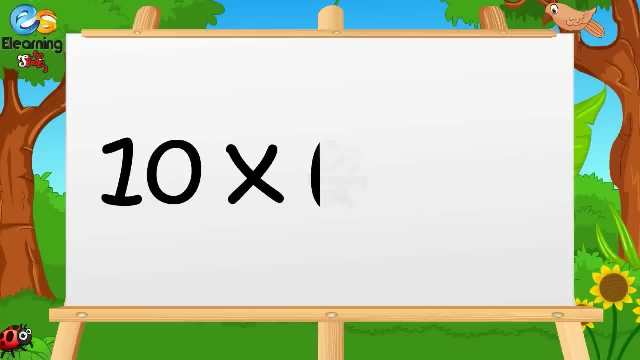 Ten, fives are fifty, Ten, sixs are sixty. Ten, sixs are sixty. Ten, sevens are seventy. Ten sevens are seventy. Ten, eights are eighty. Ten, eights are eighty. Ten, nines are ninety. Ten, nines are ninety. Ten, nines are ninety. 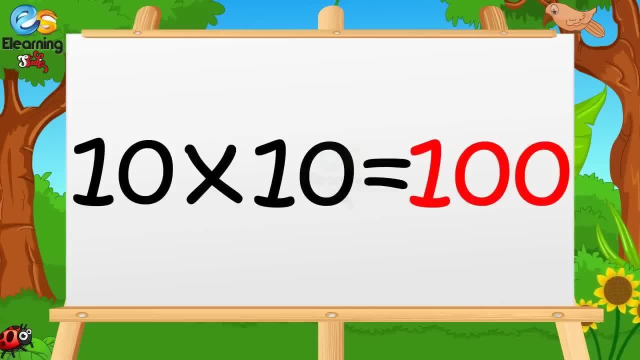 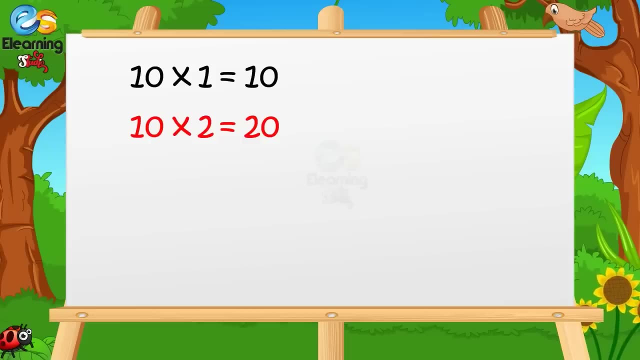 Ten tens are hundred. Ten tens are hundred, Ten ones are ten, Ten ones are ten. Ten, twos are twenty. Ten, twos are twenty, Ten, threes are thirty, Ten, threes are thirty, Ten, threes are thirty, Ten, fours are forty. 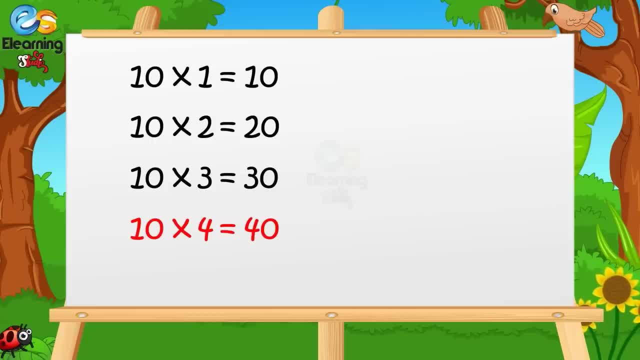 Ten fours are forty. Ten fours are forty. Ten fives are fifty. Ten fives are fifty. Ten fives are fifty. Ten sixs are sixty. Ten sixs are sixty. Ten sixs are sixty. Ten sevens are seventy. Ten sevens are seventy. 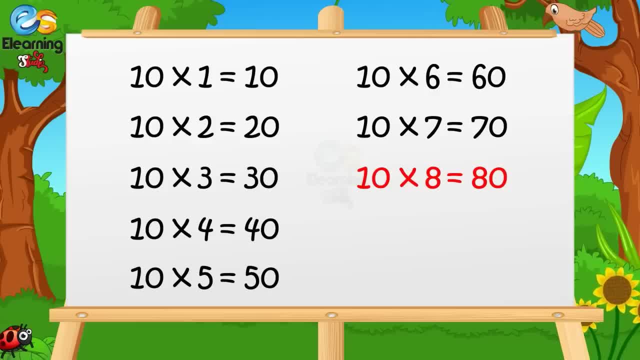 Ten, eights are eighty. Ten, eights are eighty. Ten, eights are eighty. Ten, nines are ninety. Ten, nines are ninety. Ten, tens are hundred. Ten, tens are hundred.